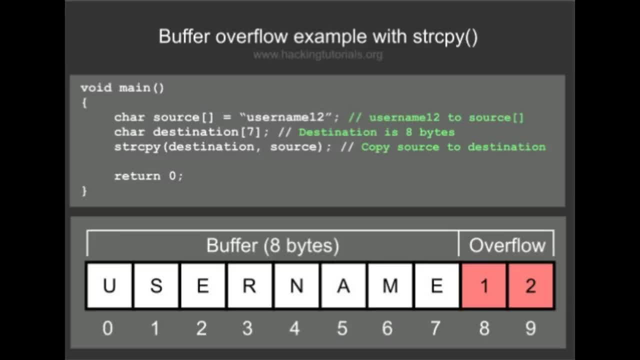 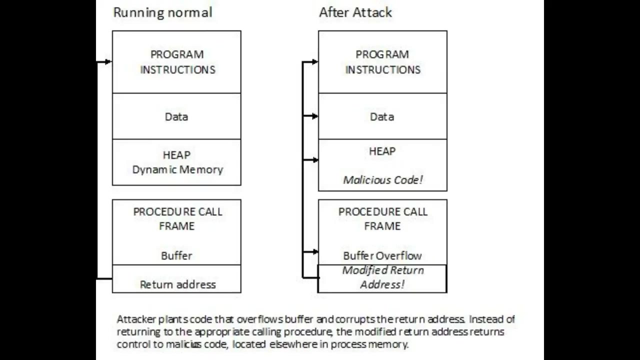 In other words, the buffer size will get overflowed and the extra input will also be processed. This is the vulnerability. This is called buffer overflow. So buffer overflow is a condition when a program writes more data to the memory than it is actually supposed to take. 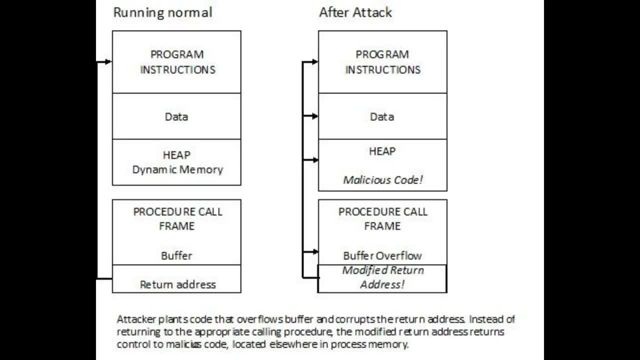 Now you will ask me What will happen to the extra input which went into the overflown buffer. What if the input contains any shell command or a malicious script or a virus command? Yes, it will go to the system itself and get executed. 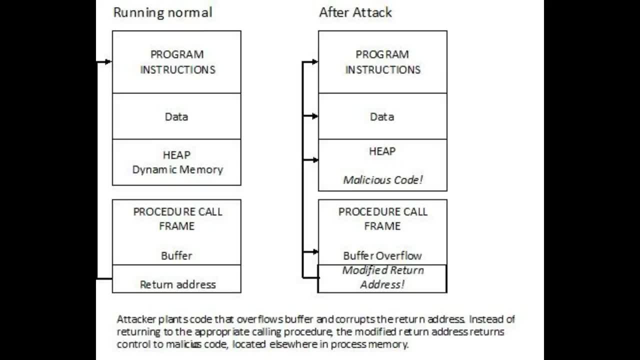 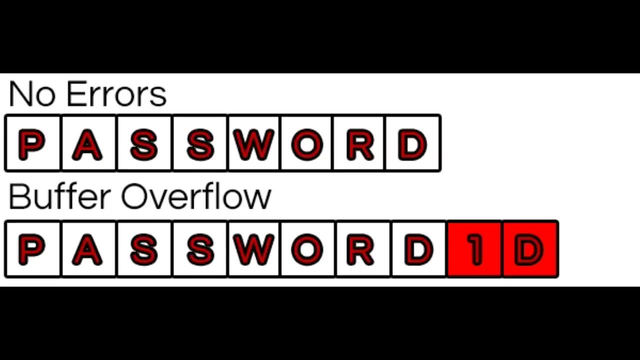 Once a script is executed on a system, the attacker can easily get access to the system. He can send a command to download the database or drop the tables or delete files, and so on. Also, due to overflow of input, the system may get crashed and ultimately go down. 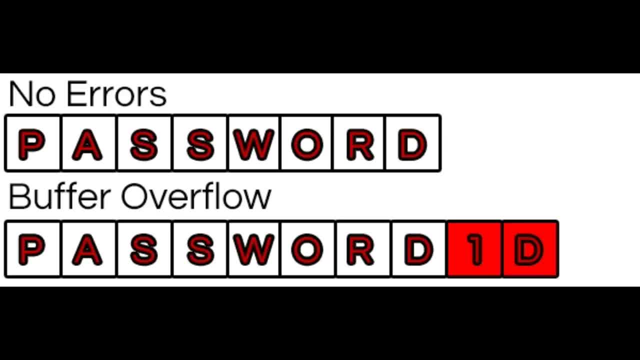 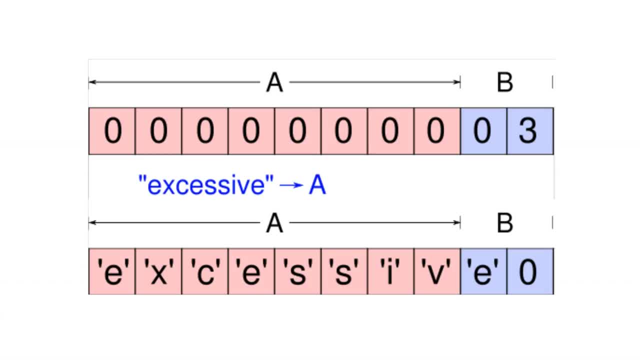 To summarize, he can challenge the integrity of the server or system. This vulnerability is exploited to target web applications, programs and servers. Buffer overflow is an example of bad programming. This vulnerability is caused by newbies and users. Buffer overflow is an example of bad programming. This vulnerability is caused by newbies or 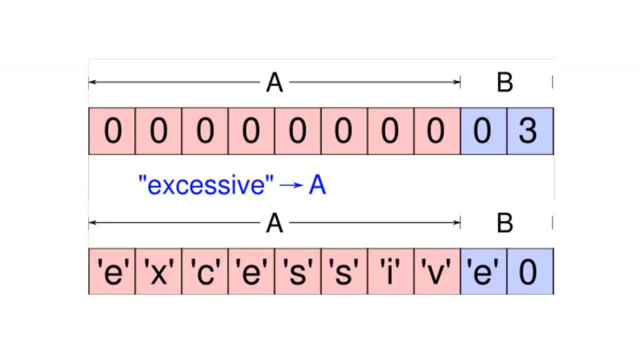 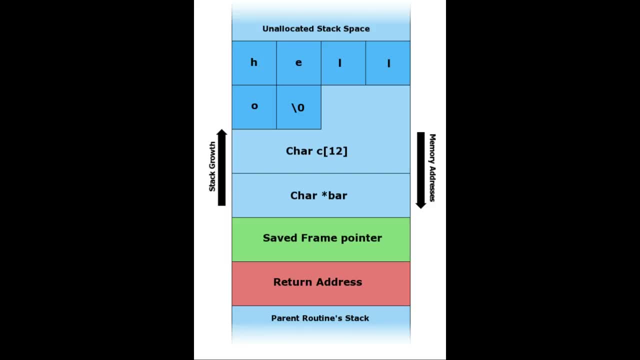 users. These users are new to programming and leave such conditions which don't raise any error. It is generally seen in C and C++ languages. New languages like CJava and Perl have somewhat reduced this vulnerability. So this was a basic overview of buffer overflow. 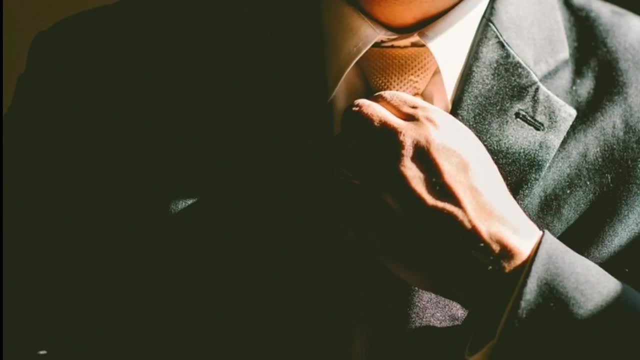 If you want a practical on this, do let me know in the comment section below. That's it for today. If you learned something from this video, streets, etc. Subscribe to my channel if you like it. Don't forget to like, share and subscribe for more videos on cyber security and technology. 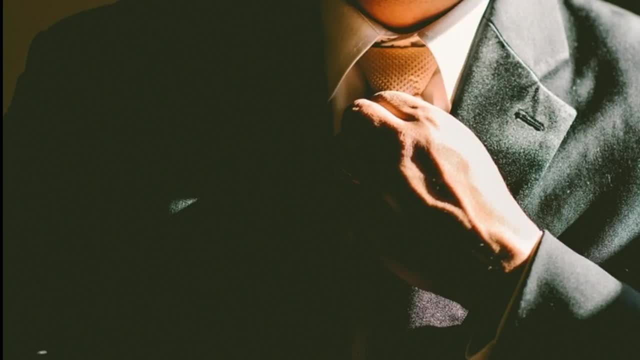 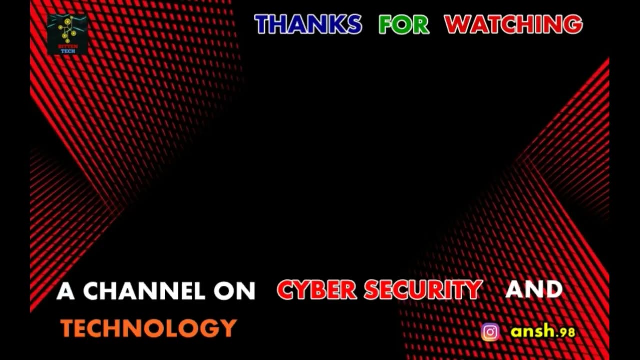 Until next video, stay tuned, Keep watching and good Bye You.